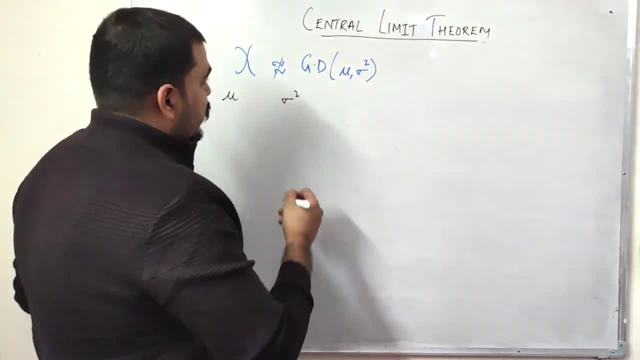 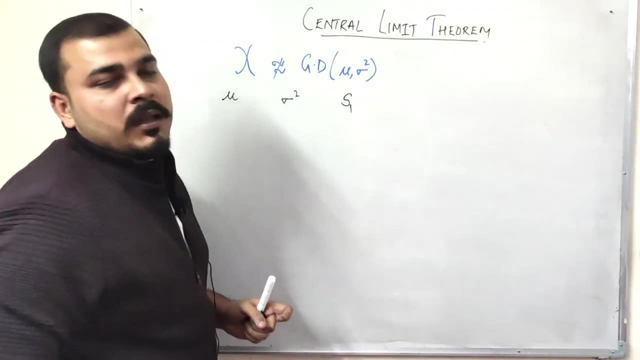 specifies? first of all, it specifies two different points. Suppose I take samples from this random variable x. Suppose I'm going to take my sample as one Now in this sample. let me consider that from this random variable I'm considering 30.. N is equal to. 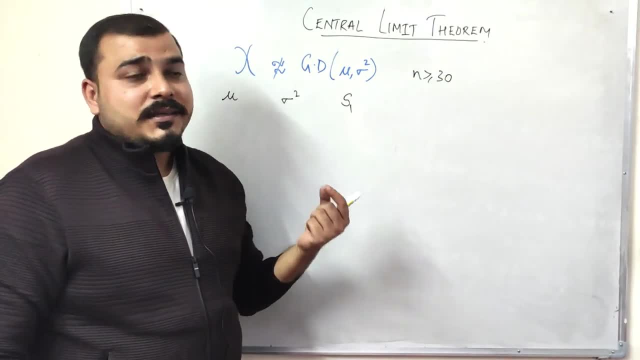 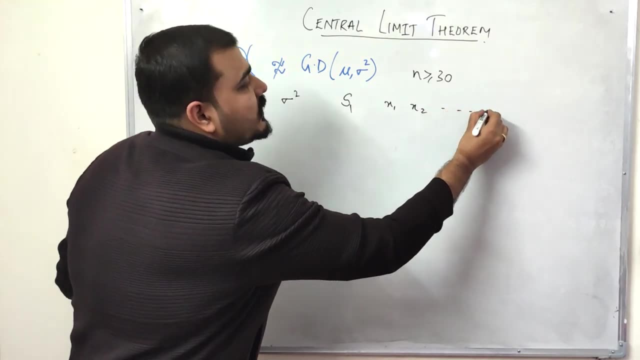 or greater than 30 data points. Okay, so if I'm considering n greater than or equal to 30 data points, So over here in my sample one, I have considered x1, x2, like this, I've considered 30. 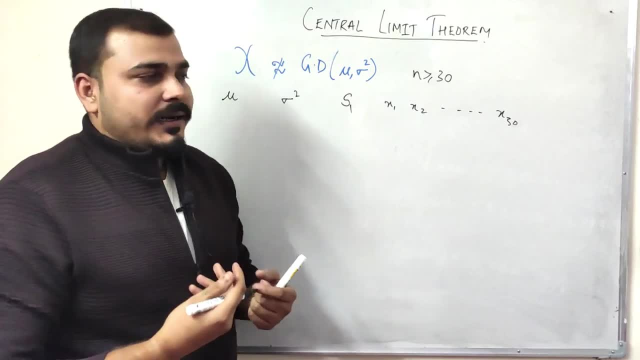 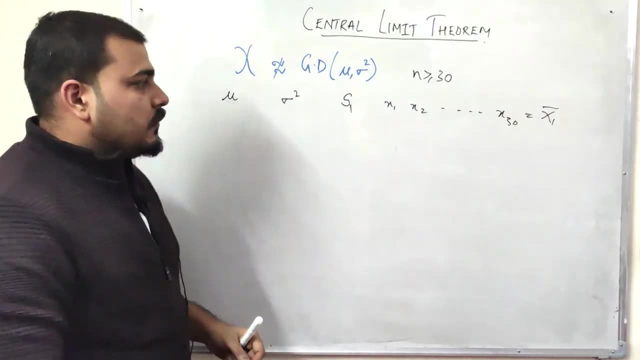 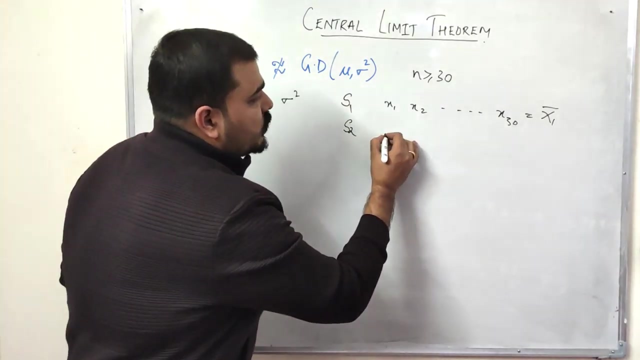 data points and I'm randomly selecting it. Okay, randomly selecting it, And for this, suppose I could find out in the next sample. I'll try to pick up some 30 data points again for my sample s2.. And this will again be over here, And let me consider this mean is x2 bar And similarly for 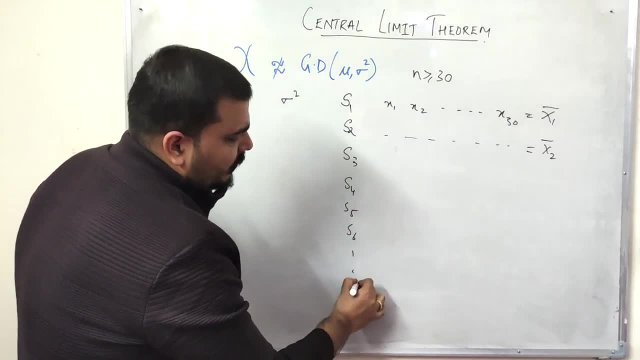 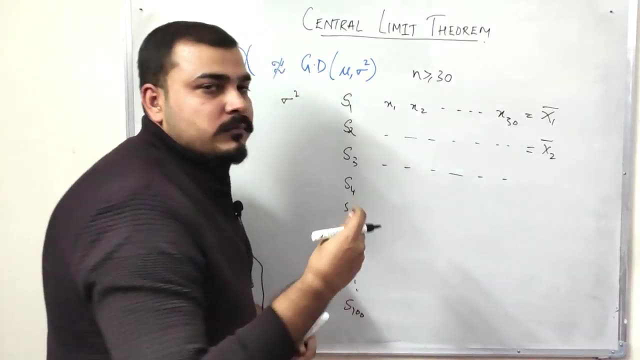 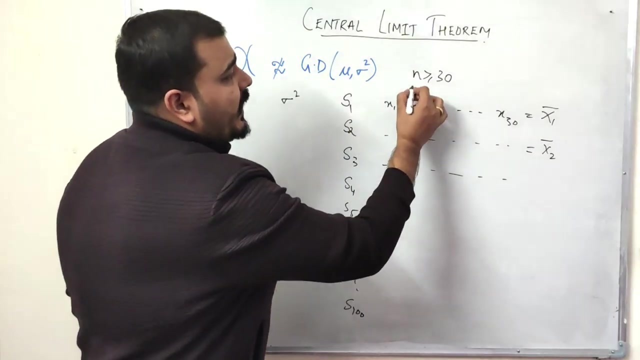 s3, for s4, for s5, for s6, and many number of samples. I have basically considered Suppose I've taken till s100 samples And every time I'm selecting 30, you know random sampling values of, I mean random sample data points from this random variable. I've made sure that my n. 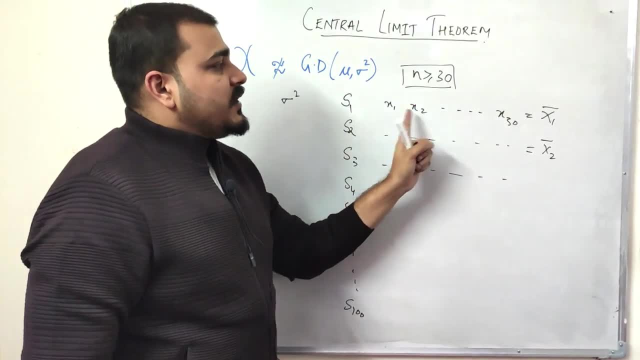 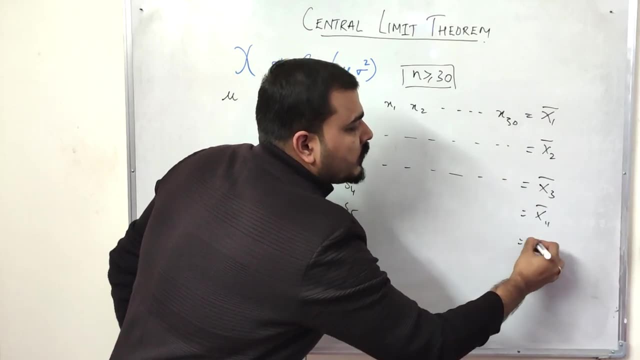 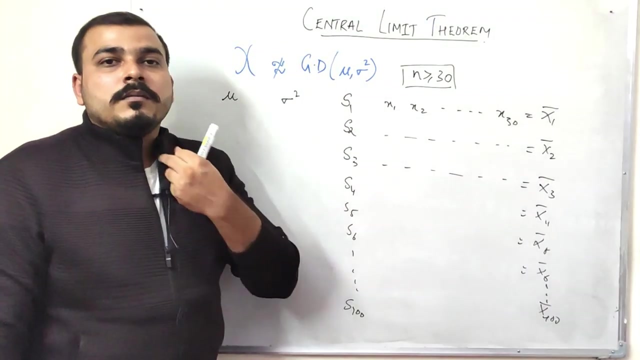 value is greater than or equal to 30. Now this n basically specifies my count of the sample values. Now, similarly, I will be calculating all my different different means. So these are all my means And I'll have till x100 mean. Okay Now, central limit theorem says that if I take 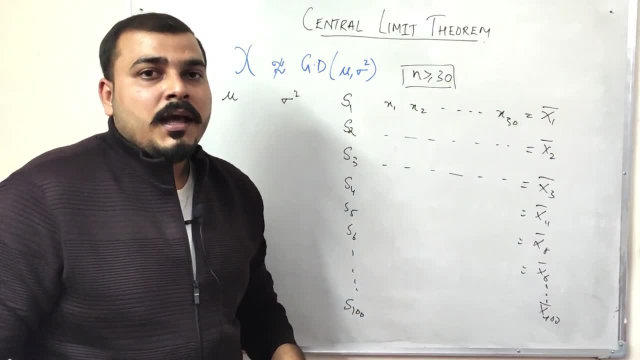 all this mean, if I take all this mean and if I try to plot them with the help of histogram, then I will be able to get x100, x100.. So if I take all this mean and if I try to plot them with, 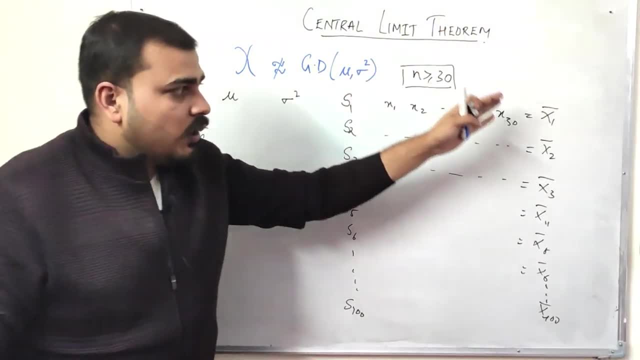 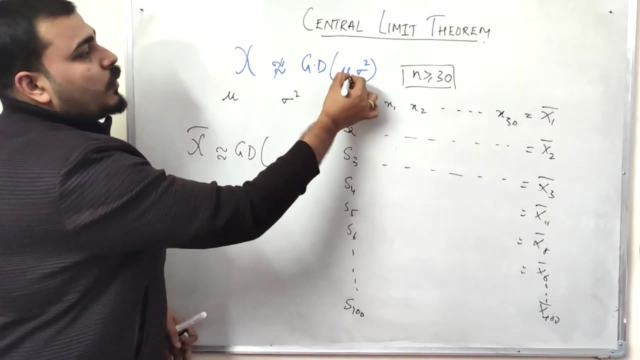 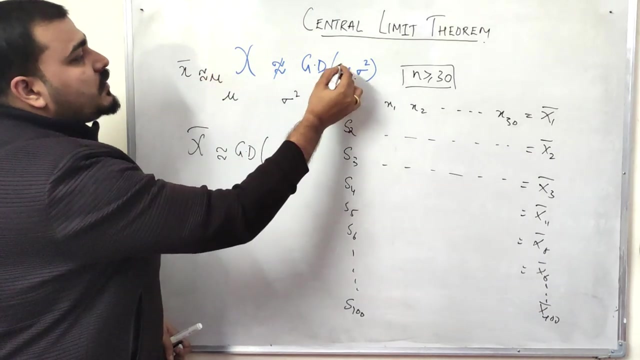 Then I will consider that this X bar, which I'm considering all the mean of my sample, will belong to a Gaussian distribution with the mean which will be equal to this mean. So suppose, if I'm taking this sample and considering X bar is my mean, this will approximately be equal to this mu, which is my population mean. 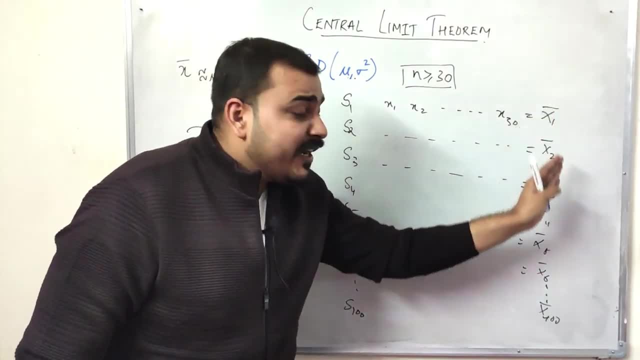 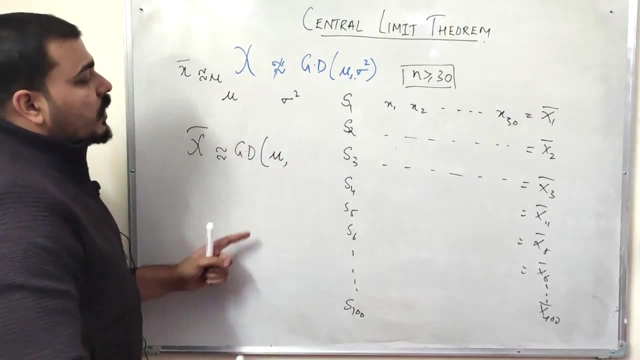 OK, so that this is the condition which will be getting satisfied by this particular sample mean over here. So this X bar will be following a Gaussian distribution with the mean which will be approximately equal to the same mean, and my variance will actually be sigma square by n.